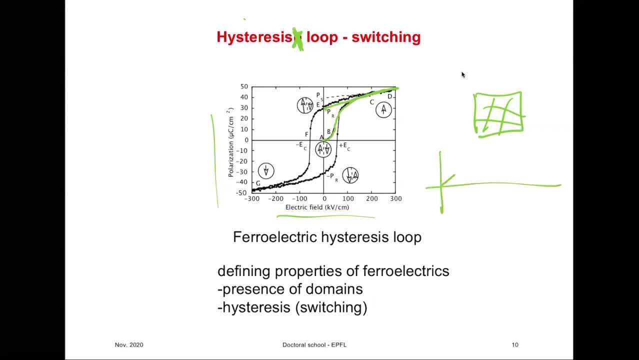 So by applying a field from zero to positive and then going back, So field, if strong enough, will start reorienting domains along those crystallographic directions that are allowed by the system And then we will see the crystal symmetry. Remember, in a tetragonal material, domains can only the polarization strain, can only develop along. 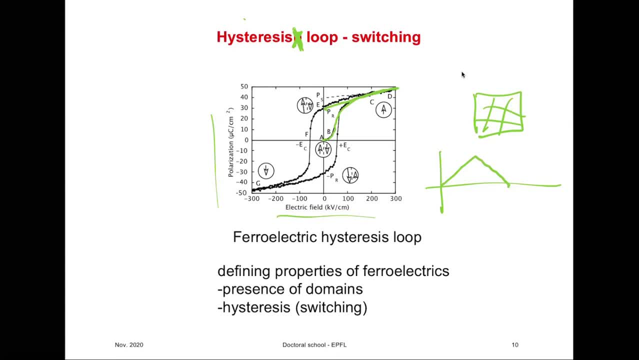 001 and perpendicular to perpendicular directions under 90 degrees. They cannot develop under other directions. That's not allowed by the symmetry of tetragonal, of the tetragonal sample. So we will, we will orient Domains as much as it is possible. 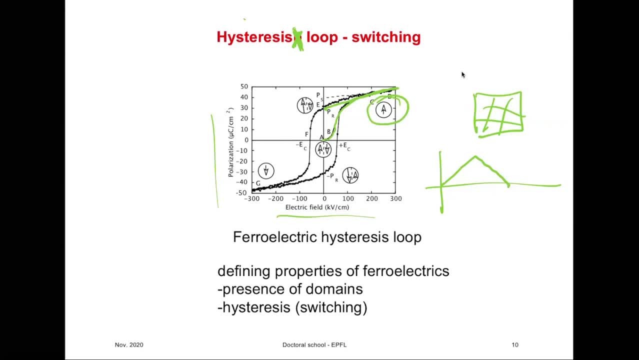 In the case of a single crystal, we can orient them and in such a way that we get a single domain: Crystal violence ceramics. It will never be possible, because of the random orientation of the grains, to align all domains in the same direction. This point here is called maximal polarization. 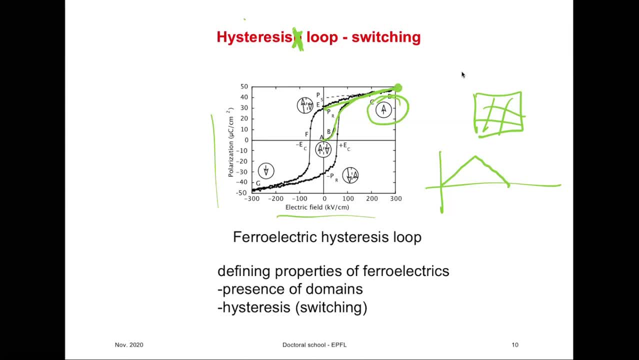 And if we go down, make projection of that to zero failed, we get the point which is called spontaneous polarization. Okay, Now, when we go down with the with the field, some of the domains will go back to to their line with the field. 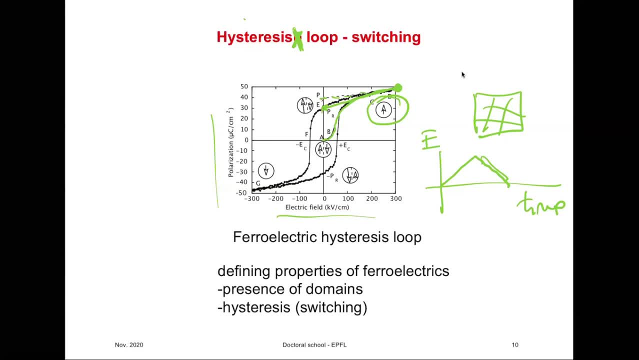 So again, So at the zero field in general, we will not reach the same point that we we will not reach the spontaneous polarization. The slope here is simply the fact that by applying electrical field, we will be inducing, in addition to spontaneous polarization, also some induced polarization. 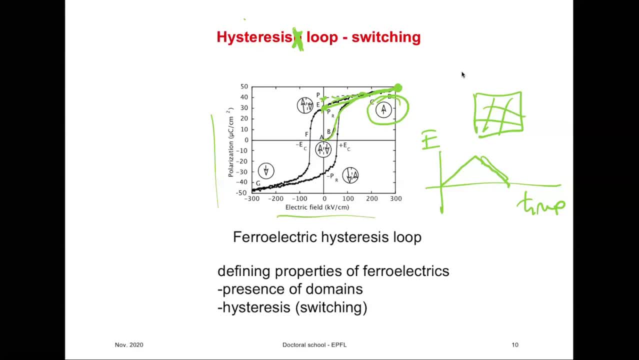 That is why we are making this projection. And then, if you start going with the field Down, Some of the domains will be oriented against the field at some point, which is called coercive field. Approximately half of the domains will be oriented along field direction and half against, 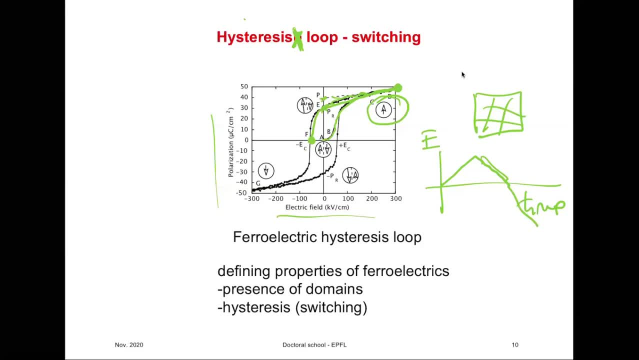 So the polarization will be equal to zero. that's called coercive field. And then we will reach the same point as on a positive field In the negative field. And then, when we further reduce field down to zero, we will go through the point of negative remnant polarization and come here to zero. 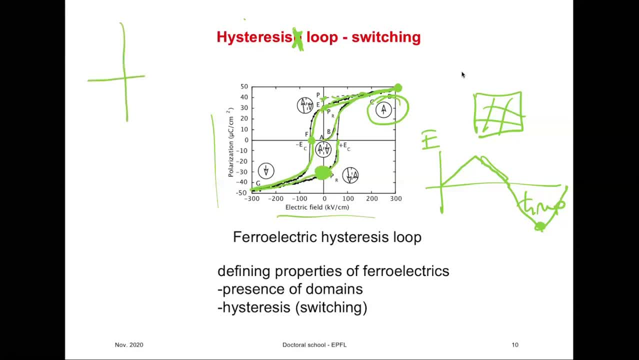 So if he had an unpauled ceramic, the failed cycle, the polarization as a function of the phase, Okay, And then if we apply field again, we will start with this point and then we would, we would do, we will do that. 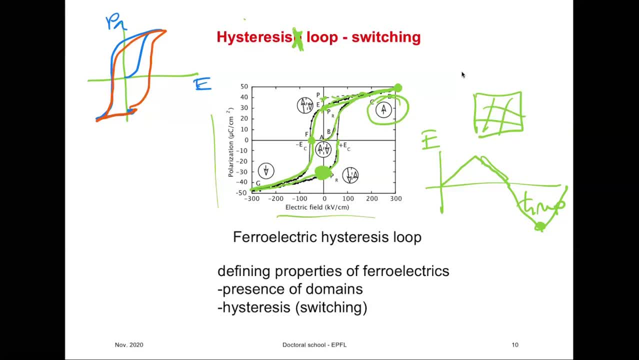 So from the shape of the hysteresis slope you can know whether the starting point of your sample was where the sample was pulled or not, And so on. So hysteresis slope Is a consequence of presence of domains, The fact that different polarization states are all equilibrium states, all stable states. 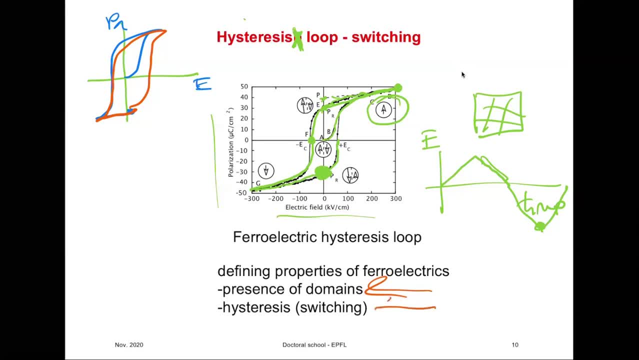 And this switching is also a characteristic of ferroelectric materials. If you have a pyroelectric material where you have Polarization but cannot be switched, You would not have. you would not have this hysteresis. So if you are looking for to to detect whether a material is for electrically, usually the sign of that is a presence of hysteresis. 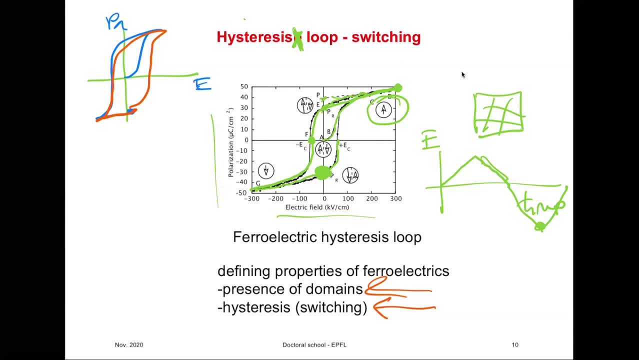 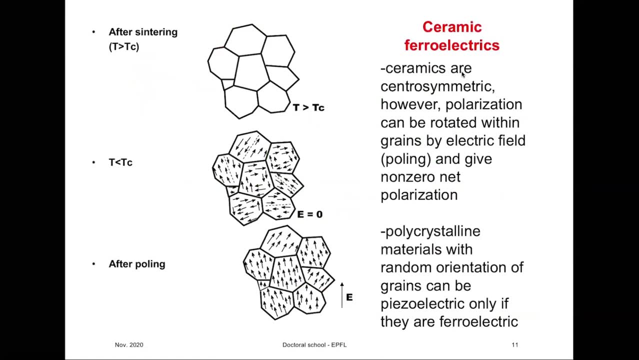 One of the signs of ferroelectricity is hysteresis. I will discuss that a little bit later. So with ceramics we have the following case. Okay, Let's say that we have a ceramic that is ferroelectric. We sinter ceramic at some high temperature. 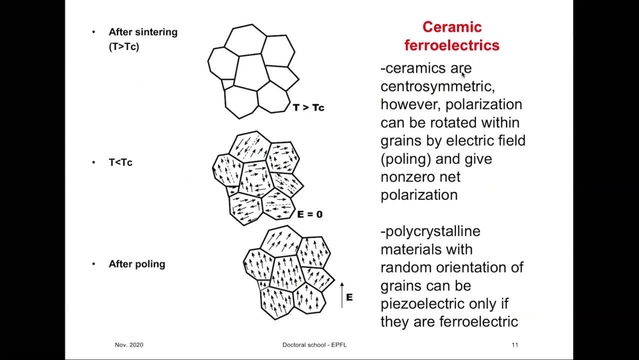 These temperatures are almost always higher than a Kiri temperature, So material is in the cubic phase. There are some exceptions, For example in a bismuth ferrite we usually do sintering below Kiri temperature. So after sintering, 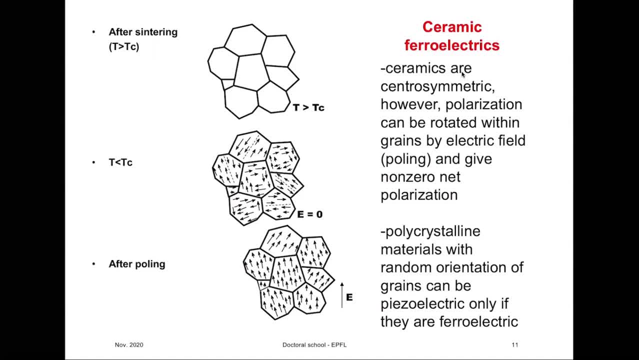 And at temperatures that are higher than a Kiri temperature, we will have a cubic grains, no polarization, And then as we cool material and we go to TC, the polarization will develop and domain walls will be formed in the material So that, because of the random arrangement of the grains, 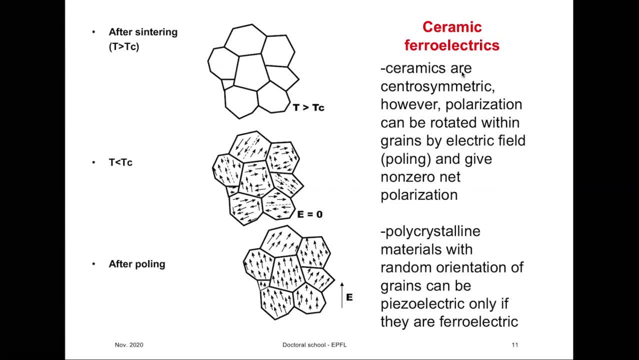 And presence of domains, the net polarization is equal to zero. So the polarization polarization is equal to zero. However, if you apply electric field, and that electric field can be applied either below TC or above TC, and then sample is cooled to room temperature, 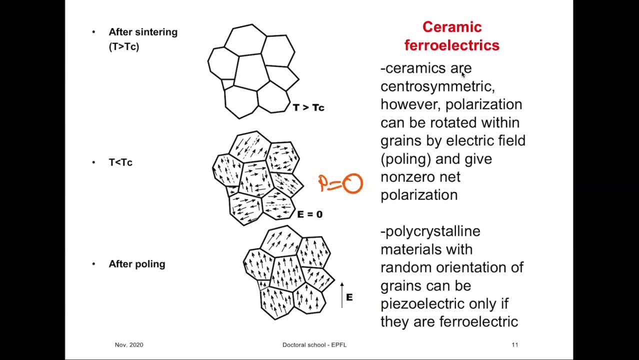 We can align polarization In grains along one of the polar directions, Since grains are oriented differently, not all of them. So for this one, C axis is here, C axis is here, And and so on. We will usually not have that. 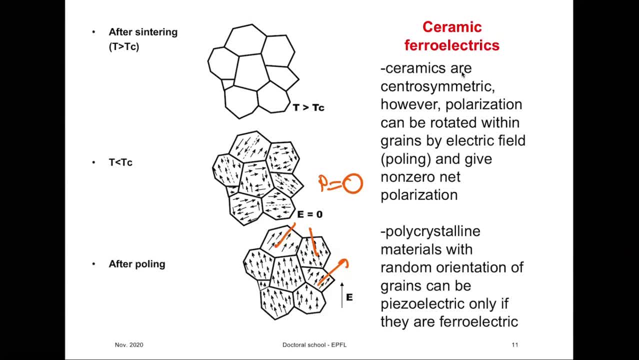 Any of the grains In ceramic are single domain And that's because there will be some Some strain in every grain due to surrounding material which doesn't have the same orientation. And while we can get rid of most of the 180 degree domains, some 90 degree domains almost always remain in a sample. 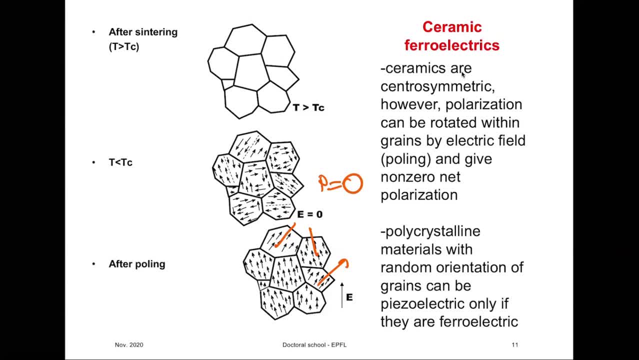 Now there are materials that are uniaxial, ferroelectric, Such as lithium niobate, in which you have only 180 degree domains, And there it might be possible. I actually don't know whether one can have a ceramic without any domains in the lithium niobate ceramics. 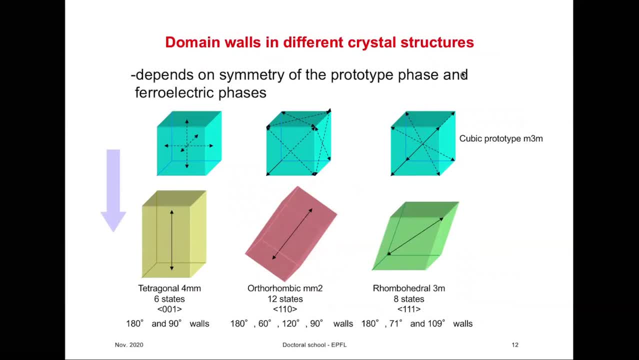 So what kind of domain walls are possible in ferroelectric materials can be determined from the symmetry Of the paraelectric phase, that's phase, non ferroelectric phase, above TC, We call it paraelectric phase, And from the symmetry of that phase you can actually tell. 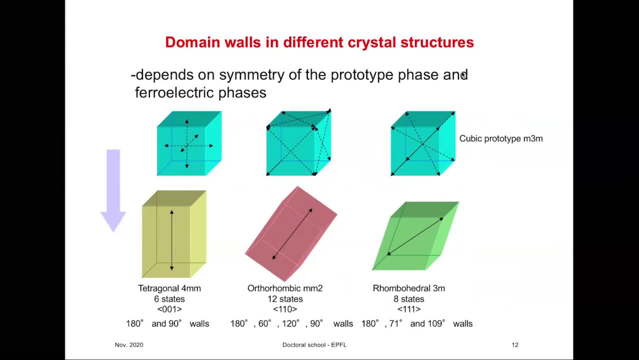 What? by the symmetry of the material, what kind of domain walls you might have. That doesn't mean that all those states will develop, But those are possible, Possible states by the symmetry And I have given previously. I'm not going to go back to that. 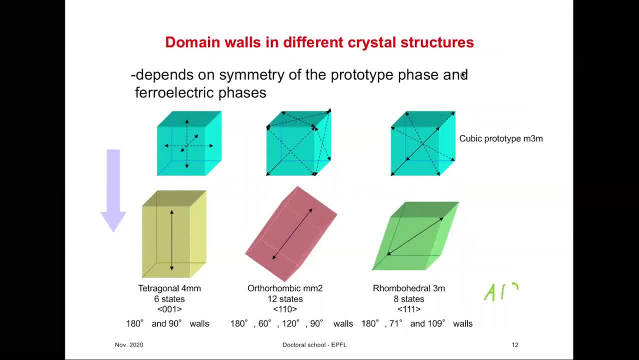 But there are two papers by Aizu in which he derives, with all for all crystal symmetries, What are the possible domain states that one can get. So you can find it, Those two references on one of the previous slides. So if you look at a cube, 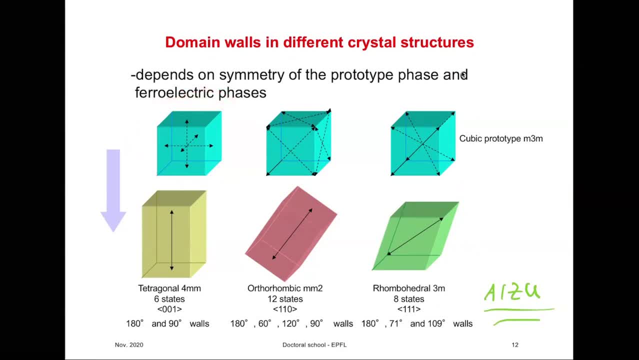 Here We are looking at symmetry, different symmetry elements, And we see that we have these. So these are along the crystallographic axis. That would give us a tetragonal phase, For example, if you start with the M3M phase. 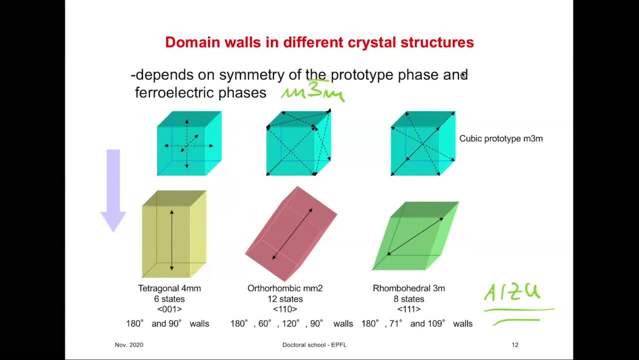 We can get a cubic M3M, M3 bar, M phase. We can get tetragonal phase 4MM With six states And that will give you 180 and 90 degree domain walls. Then you can also look at these. 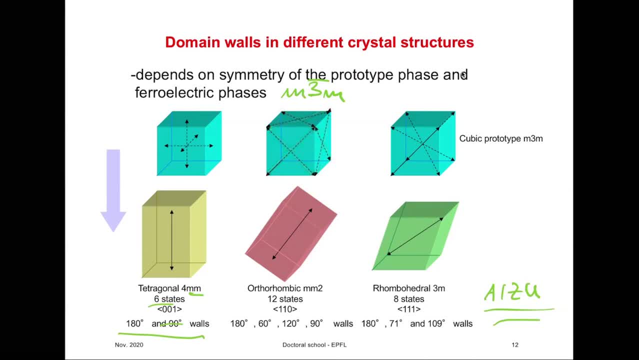 Elements along Side diagonals Of the cube And that can give you The. And then you can look Symmetry with respect to diagonal of the cube And that can give you a number Three, M phase with eight possible domain states. So here we have 12,, six along sides and plus minus. 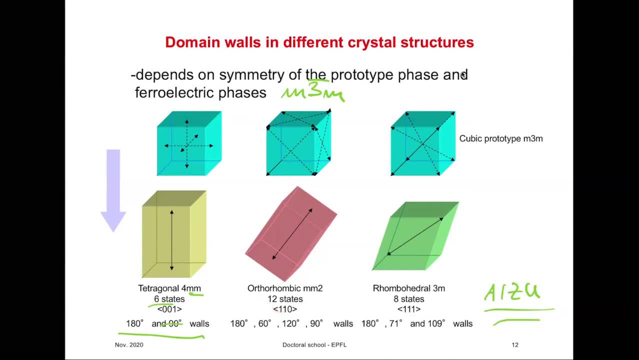 because of 180 degrees, that gives you a total of 12.. And here we have four diagonals: body diagonals and then plus and minus 180.. You can get 71,, 109, and 180 domain walls. It is possible that M3M also gives you monoclinic structures, which have been discovered in. 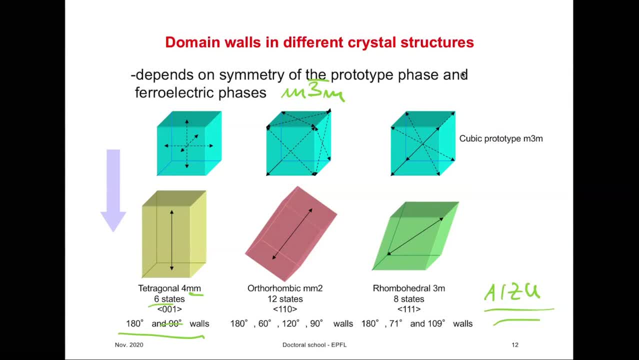 many of these more complex ferroelectric materials not in a barium titanate, For example, lead titanate, barium titanate. both have a M3M structure, But this one gives you only M3M cubic structure, but this one gives you only. 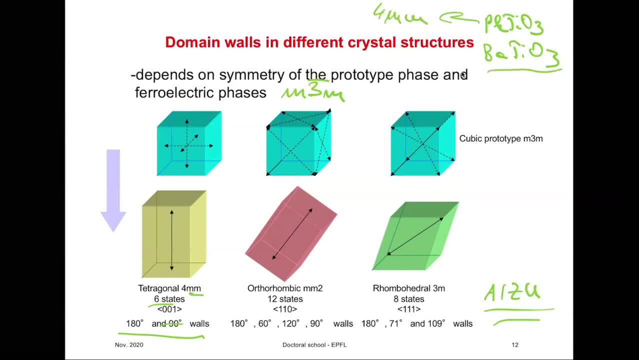 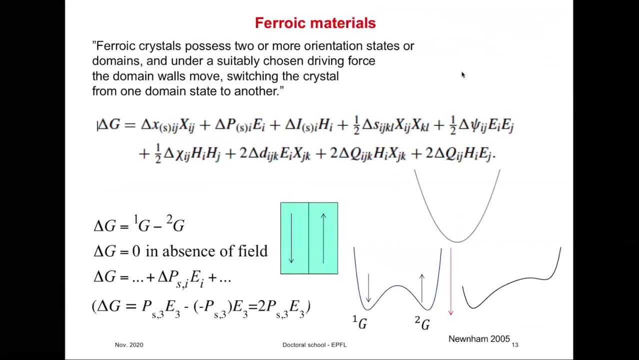 4MM ferroelectric phase, while this one gives the three tetragonal, rhomboidral and orthorhombic phase. Domain walls are intimately connected to what is called ferroic materials, and I just want to give you a word on that, because it's a very popular topic now. 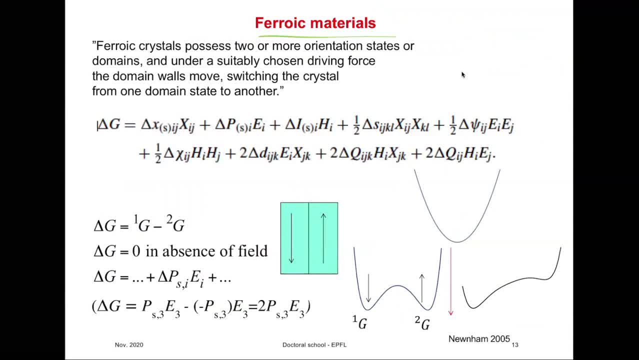 People are looking for a multi-ferroic materials. Those would be materials that are at the same time ferroelectric and ferromagnetic. And what would that mean? That would mean that you can affect magnetization by electric field or polarization by magnetic field. 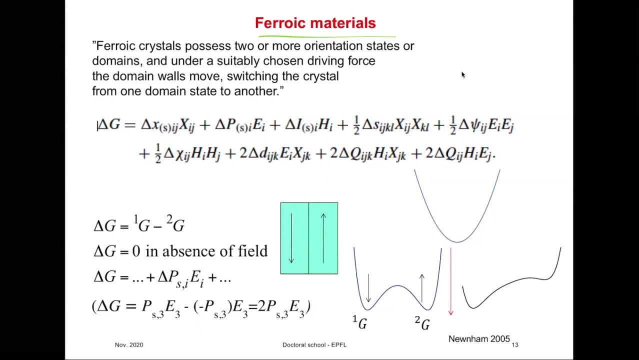 And that would be really interesting from the point of view of devices. Such materials have been discovered, but they are usually multi-ferroic at very low temperatures. Some of them are multi-ferroic at room temperature, such as bismuth ferrite, but it is not ferromagnetic but 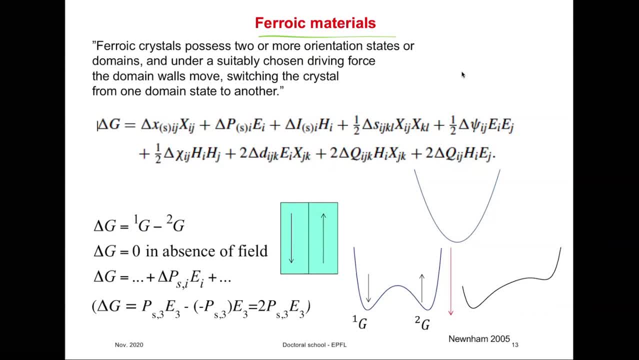 anti-ferromagnetic and so that's not so useful. So basically, any material which develops domains, either electrical, electric and electric domains, or magnetic domains or elastic domains, is called a ferroic material. So, for example, barium titanate is a multi-ferroic material, It is ferroelectric. 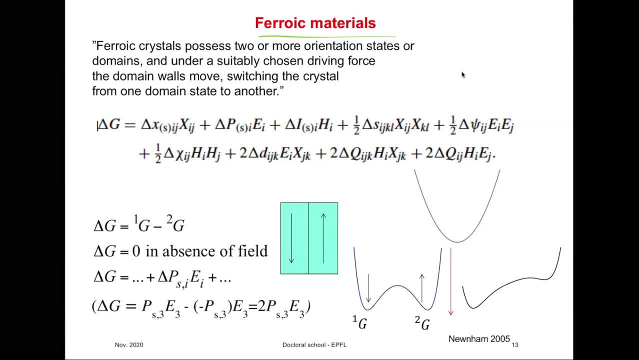 and also ferroelastic because it has this strain that develops at a phase transition. However, its 90 degree domains, which are ferroelastic domains, are also at the same time ferroelectric. So it is a ferroelectric, ferroelastic material, but it has purely ferroelectric domains. 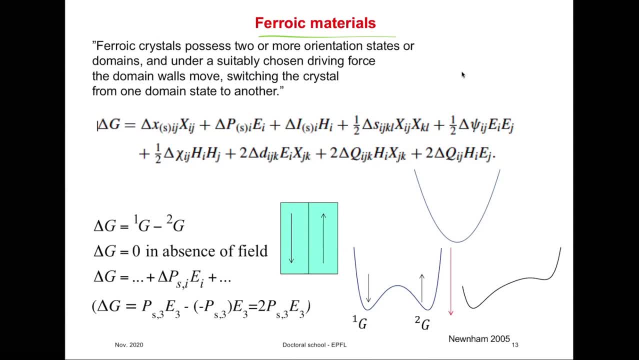 and ferroelectric ferroelastic. It doesn't have purely ferroelastic domains. A material that is ferroelastic without having polarization is, for example, zirconium dioxide. You can learn about this from Newnham's book. there is a whole chapter on ferroic materials and basically 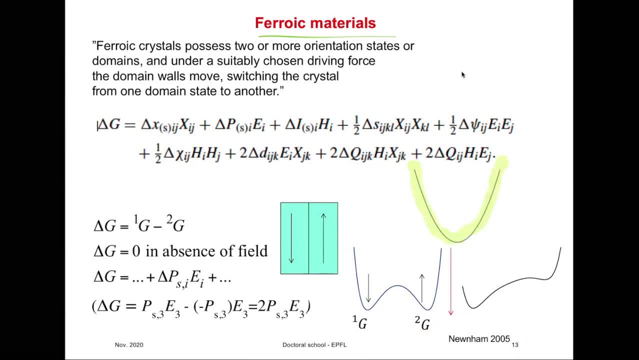 the treatment is the following: You have a cubic material- okay, there is no polarization- and as you go through the phase transition through TC, you develop these two, So polarization is zero here. then we go into ferroelectric phase. we have two states of polarization which are equivalent. 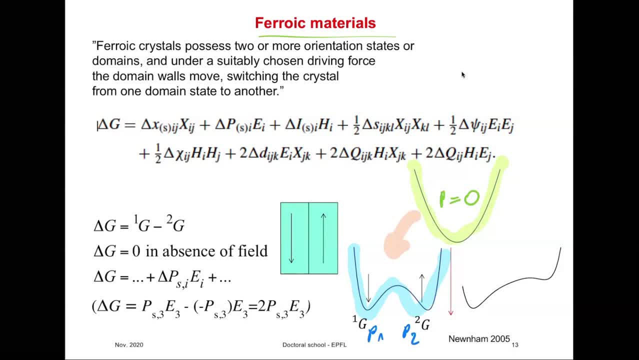 but different directions. Those two states have to differ somehow, And then when we apply external electric field, we are introducing a symmetry between these normally equivalent states. They are no longer equivalent. One of them is preferred within the mapped experiment. The other states are: more or less interrelated. So the Kurdish argument. we have an interesting expression for when we are applied an external electrical field. culturally we have stronger polarized states. they are more or less equivalent. then of course, their corresponding ethericic fundamentalism of the 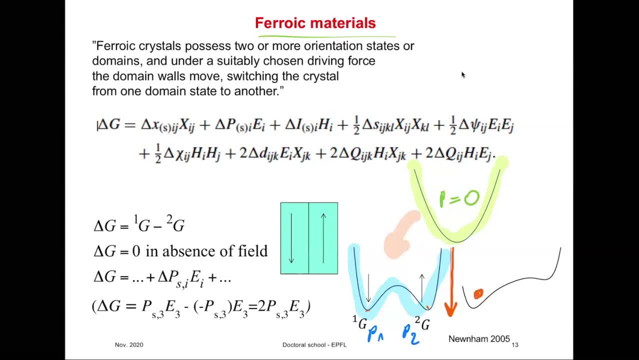 expected consequences, but these are different. And then, of course, the essence of power, Scroll included, sounds, drink, jigger, and so Batman, for example, recalls Extranet language, and so, basically, music comes from the, with respect uh to the, uh to the other. okay, so this state is preferred to this one. it has a 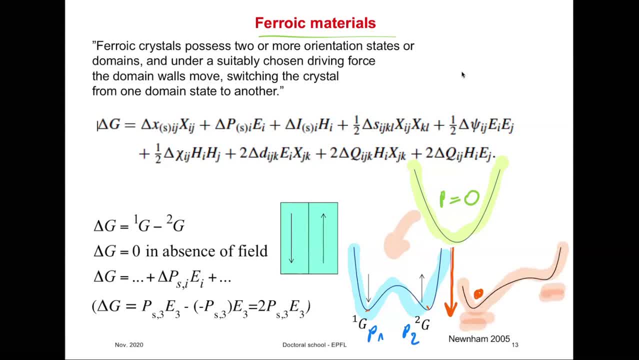 lower energy and the difference in the energy between these two states, uh, is a driving force for moving domain wall. okay, so if you had a, if you had a two domain walls, one of them, uh, polarization, looking down while looking up, if you apply electric field in this direction, uh, this, 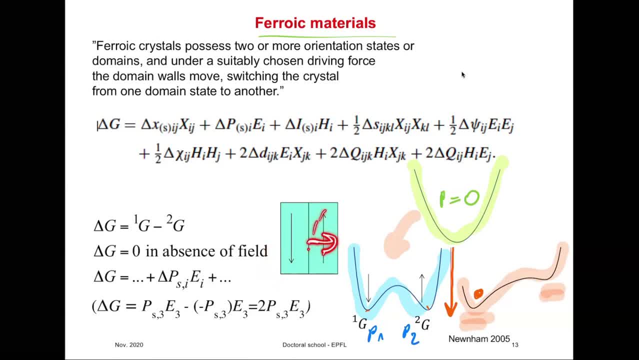 domain here. we switch that. we say that this domain, uh, polarization in this domain will switch. and we say that this domain will, a domain wall will move, uh, to the right and you can actually observe it in a microscope. uh how, uh, how it moves. i have some films, but it was challenging to prepare. 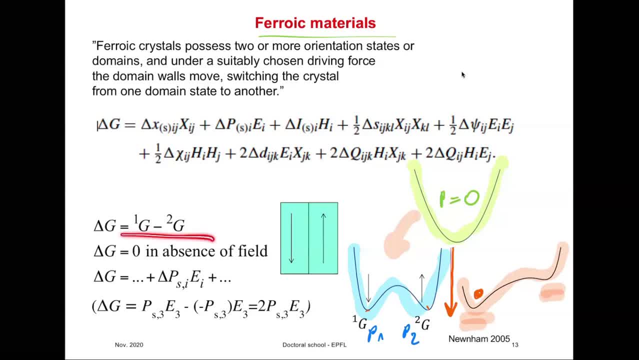 it for this. so, from these differences in uh in a state, in a polarization, strain, magnetization and so on, uh is what defines uh under, under external fields, is what defines spheroic materials. and then you have uh, uh, for example, uh. ferro b elastic uh. 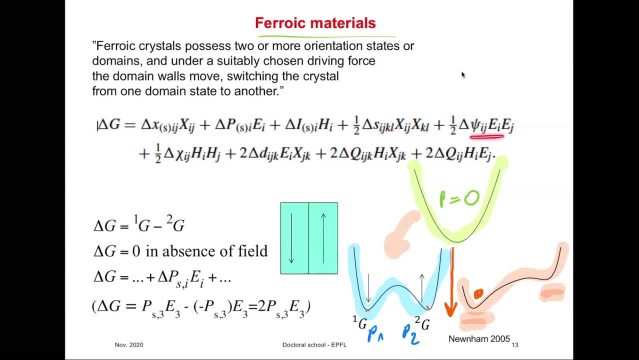 this is a different in elastic coefficient. you have ferro b electric, ferro b magnetic and then you have uh, ferro, uh, uh, i think, b electro elastic, where you have a difference in the paizoelectric constants between two different states and so on. so you can read this in, about this in unam's: 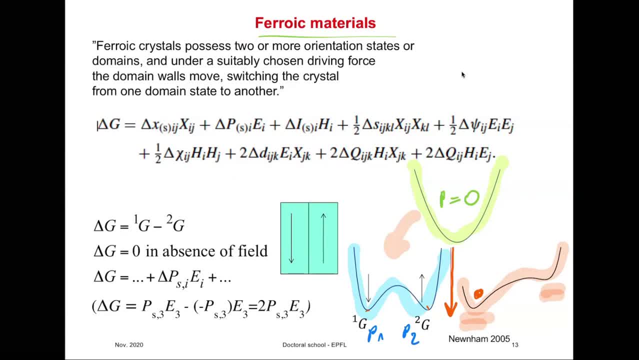 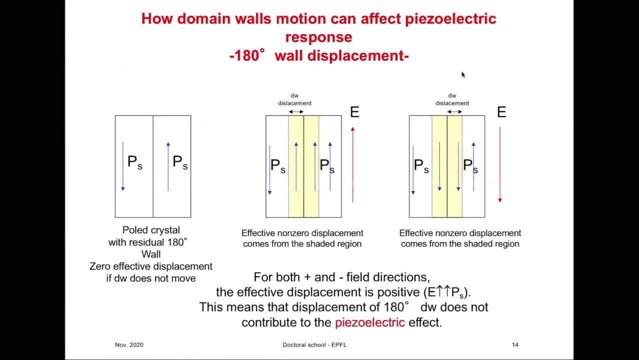 book. but there is a energy reason why uh��some some uh SPEAKER that the uh Çok um. we think the German dynascal deep end uh bats look like in the book of Nothern history and so on. uh and uh. so a lot of whom, uh, even so a lot of them uh saw a in ah, perhaps, as 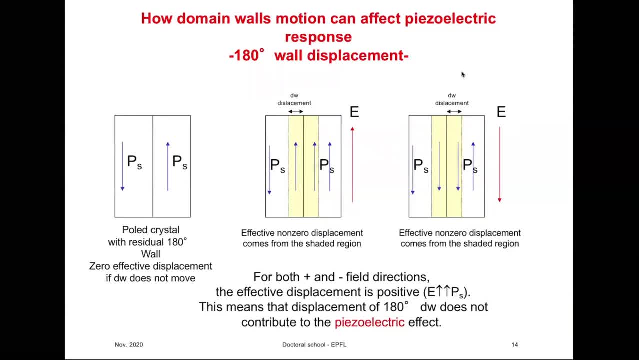 em an important– some reason why this is not completely consistent, but try to follow the general idea. So let's say we have a crystal which gives us two domains, one which is polarization going down and one where polarization is going up, And we now apply electric field in this direction, which means that we are energetically preferring this orientation of polarization to this one. 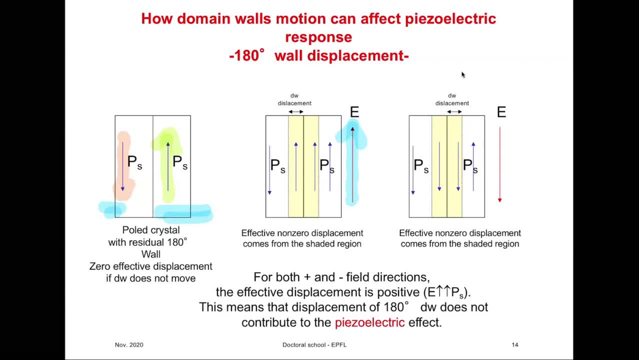 That means that this domain wall will move, So it will move on expense of this polarization. So we will get that. now the positive domain is this and the negative domain is this. Now let's see what's the difference between these two states. 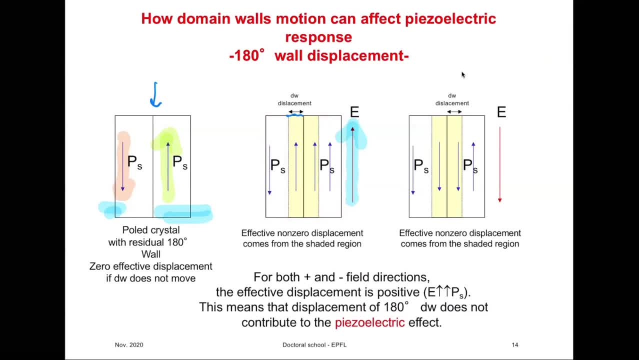 Well, the difference is this yellow, this yellow part. OK, That's the difference between this state and this state. These two give you, in total, zero polarization, But what you have gained in a polarization is this, is this volume here. So the new part here and the difference of them, the effective polarization is positive polarization is this one. 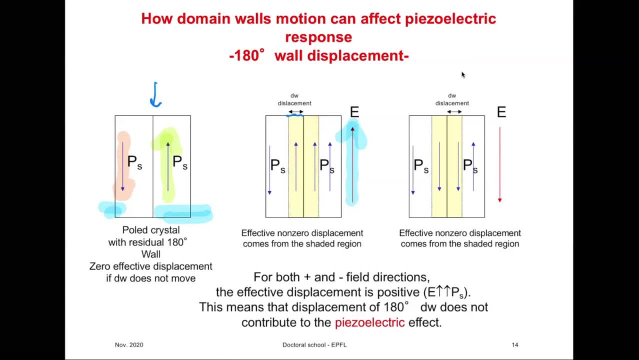 If you now apply field in the opposite direction, we will move this domain wall in this direction. So it will displace like this: Again: this part and this part. cancel, if you want. And it's this central part which remains as effective polarization in the material. 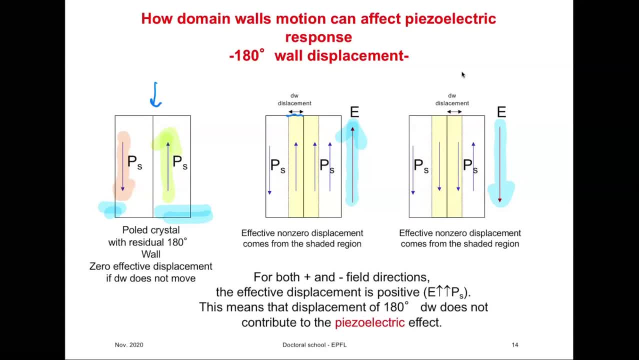 But look what happens in both cases: Final polarization And the field have the same direction. OK, Nothing has changed. And you know what happens in a piezoelectric material. In a piezoelectric material, when we turn field upside down, sample goes from extension to contraction. 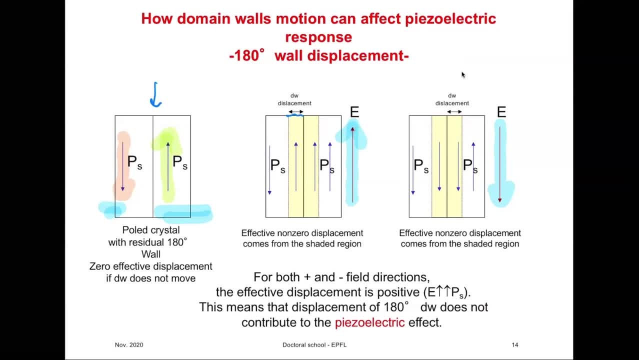 And here, since the field is along polarization, it will, for example, expand, expand it. And in this case, field is still In the same direction as a net polarization and will also expand it. So, application of the field: in both cases: expand crystal. 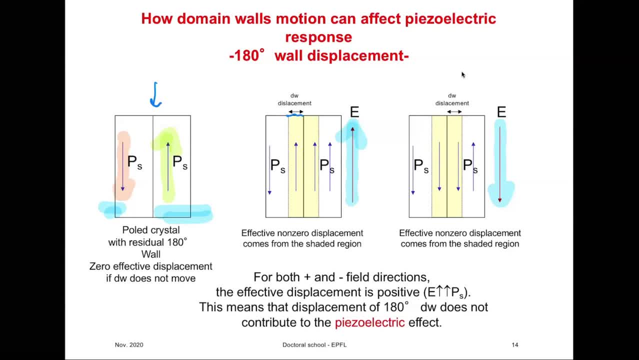 That's not piezoelectric effect. So movement of this wall didn't change piezoelectric effect. Of course, if I apply additional AC field, that would be different, But considering just this field that we are applying, under which we are observing domain wall movement, 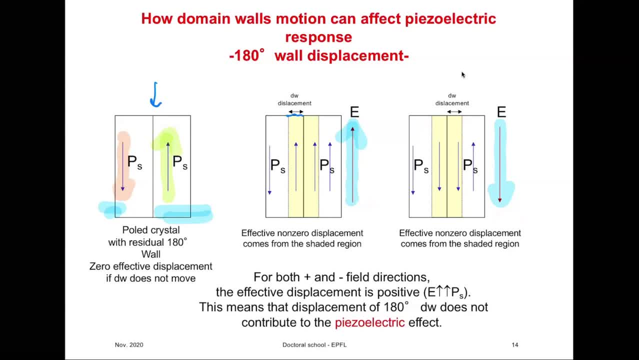 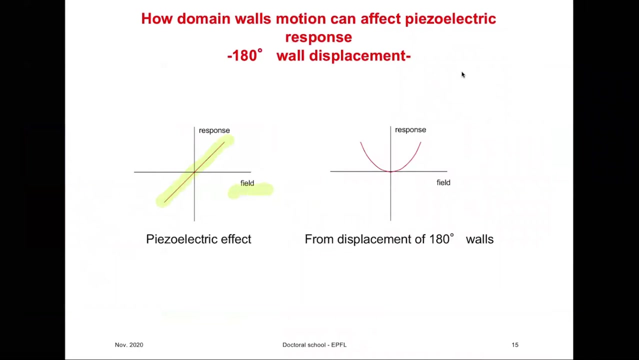 We don't have contribution to piezoelectric effect. So displacement of 180 degree domain wall does not contribute to the piezoelectric effect. OK, So piezoelectric effect requires this: When field changes direction, that response changes direction. 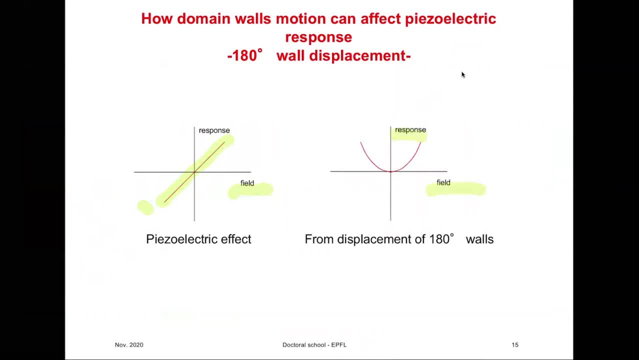 What we have from 180 degree domain walls and that for both directions of the field we have the same either positive or negative response. So from displacement of 180 degree domain walls we have, we don't have, piezoelectricity. What is this? 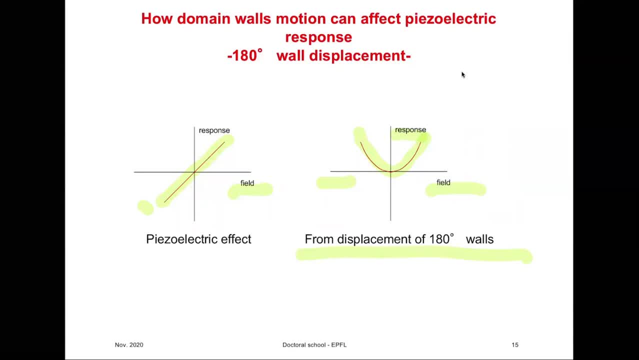 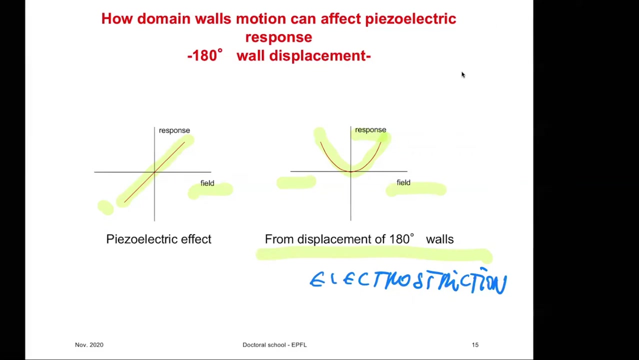 Well, if you remember previously, when we were discussing higher order terms, this looks just like electrostriction. OK, So it looks as though 180 degree displacement of 180 degree domain walls would in fact contribute to electrostrictive effect. Now let's see 90 degree domain walls. 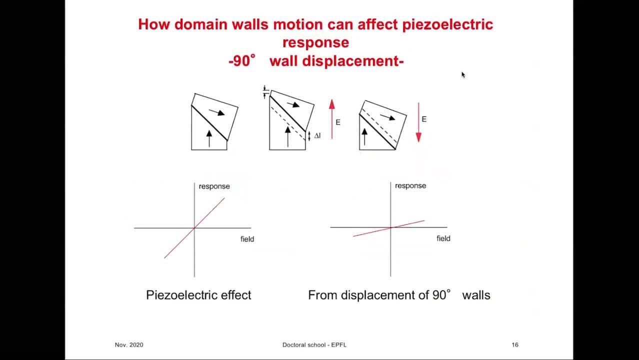 What happens? What happens there? Well, I'm exaggerating a little bit here The formation of the crystal. The two domains are never and it comes geometrically. I'm not going to go into that. but you cannot have 80, exactly 190 degree angle between polarization, two domains. 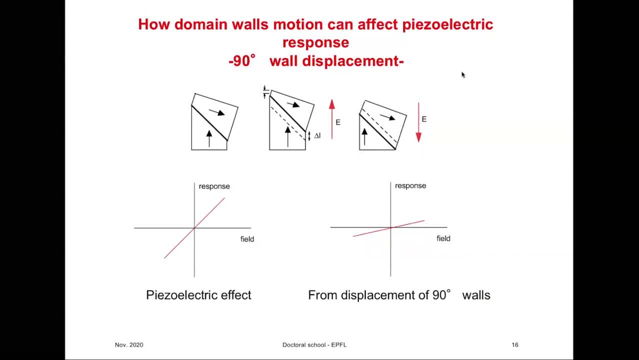 You have seen the look at these pictures that I have given before for a high resolution, atomic resolution domains And you will see that there is a small. The tangle is not exactly 90 degrees, but a little bit, a little bit smaller. 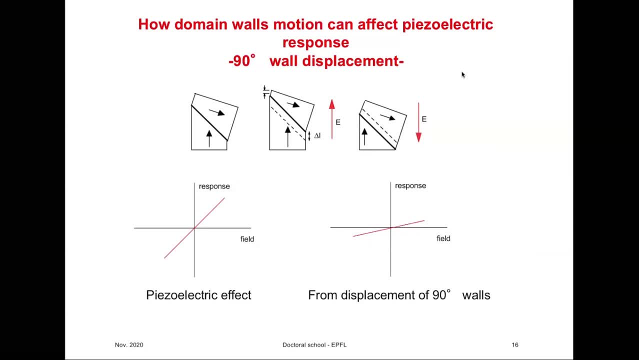 I think about half a degrees, And that's just to make possible continuity of the lattice. Now I'm exaggerating here. but imagine that we have a crystal in which there are there is one domain wall. Now, when we apply electric field in this direction, 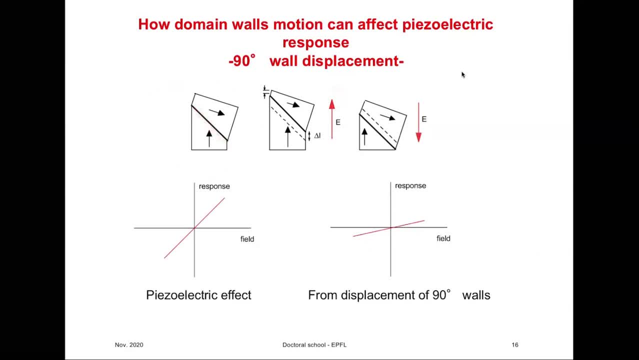 This domain wall will move on expense of this one and the crystal will change its dimension, its size, by some factor, delta L. If I apply field in this direction, then I will move this. I will move this domain wall Down By the. 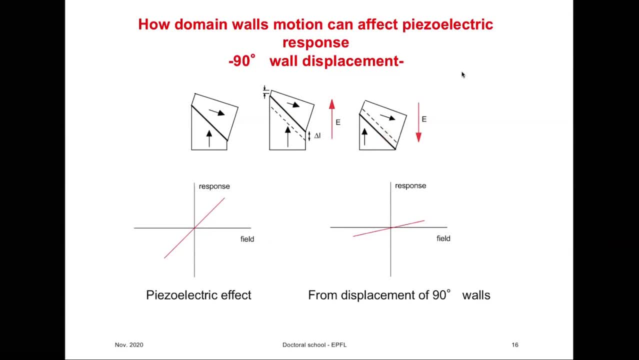 By the same, By the, by the basically same amount, but it will be minus delta L with respect to this one. So I'm not drawing this nicely, Something like this, where this is above this line and this is below this line. I think the actual drawing is better than what I can do with the pen.